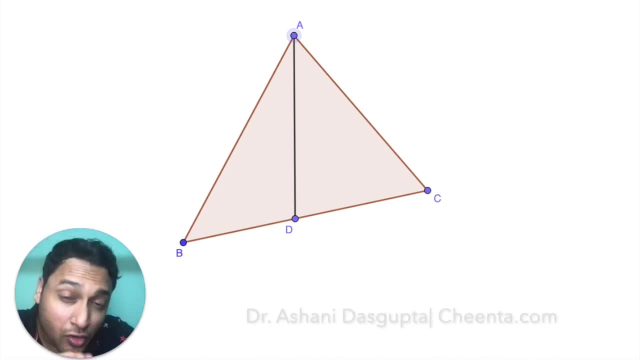 Let's join A- D. We will draw two circles. One is through A, B, D, and then we draw another circle which is through A, D, C. Okay, these two circles are drawn. Now let's mark the point E and F, which are the intersection points of the two circles with A- C. 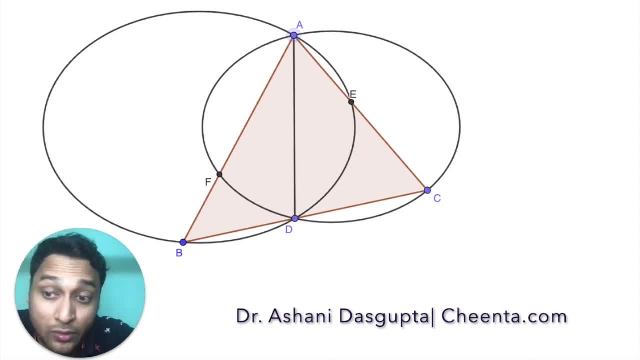 and B D. We'll also draw the circle through A, B C, The circumcircle through A, B C. Now let's join C, F and produce it to hit the red circle. Red circle is the circumcircle of A, B, C, and let's 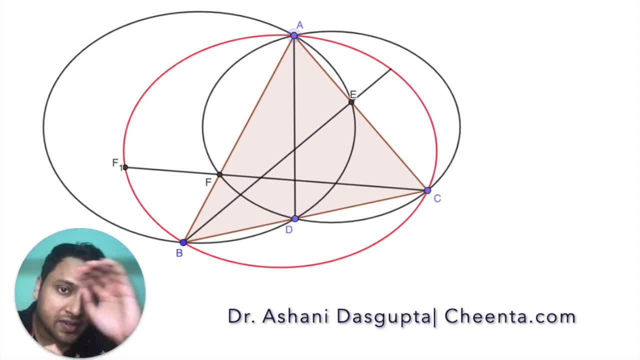 join B, E and produce it to meet the red circle at E1.. And let's extend A, D to meet the red circle at D1.. All right, now we will draw two triangles: D, E, F. That's the first triangle and the other. 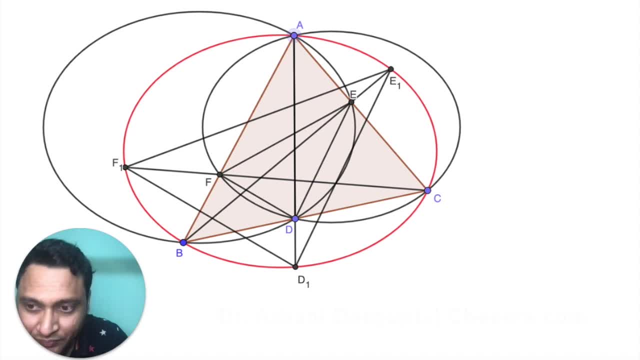 triangle is D1, E1, F1.. And finally, let's mark the in-center of D E F, which is I. Now the diagram is ready. You can also draw this diagram in your notebook and then come back to this video where we will discuss the solution, But I will do that in a 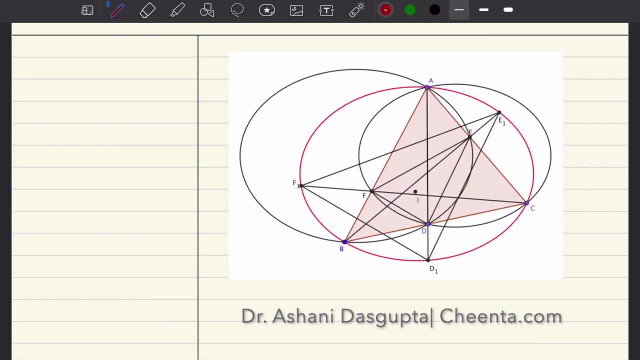 sequence of hints. so that you can do it with me, Let me first tell you what the goal is. Suppose I1, is the in-center of D1, F1, E1.. I have not drawn I1 in this picture yet. So if I1 is the in-center, 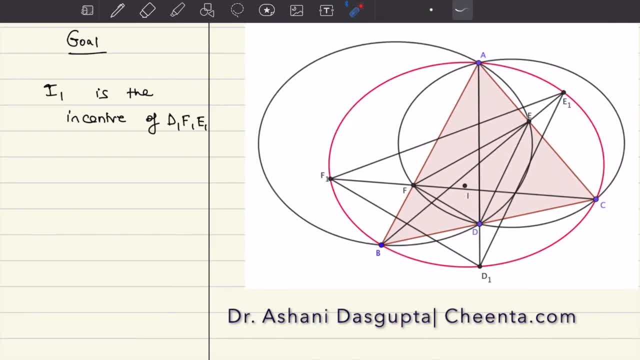 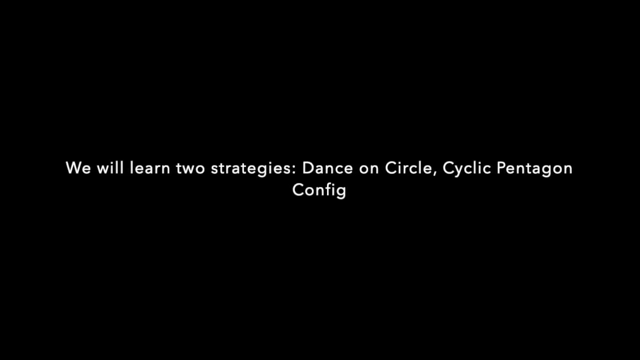 of D1, F1, E1, this triangle. our goal is to show us that E? F is cyclic. This is the main claim of the problem, That is, structures E F. wherever I1 is E1 equals I2, which means the center of sinθ ispectrator. 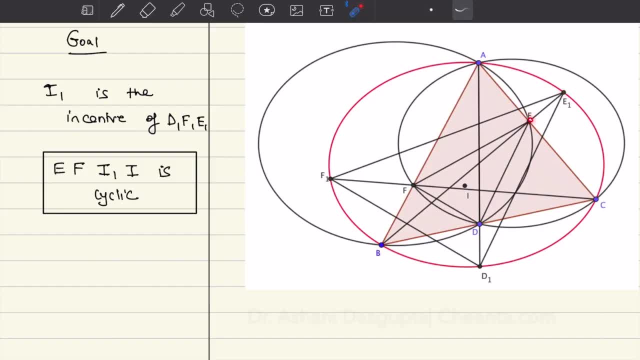 Now the answer is E2.. I2 equals I2Ω. Let's switch back and watch the diagram again. this particular quadrilateral is cyclic. that's what we want to show, and we will do this in a sequence of steps. so, as a first step- and this is a hint again- step 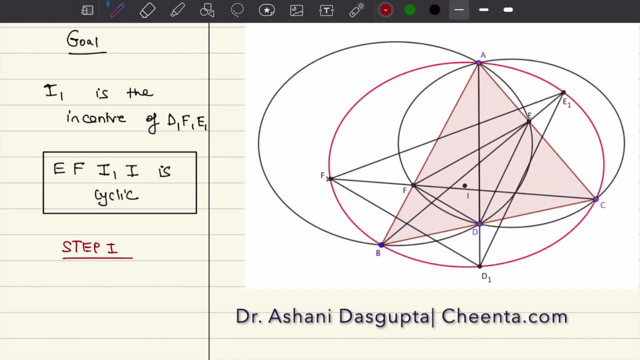 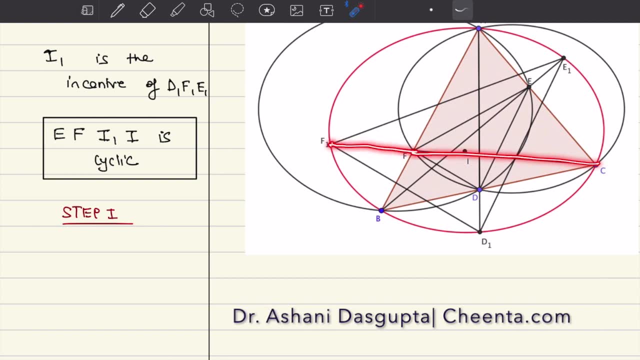 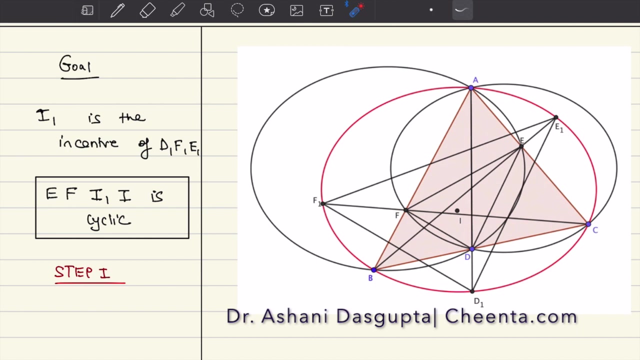 1, I would say show that CF is actually a bisector of F1 and BE is actually a bisector of E1. this is quite incredible. you join CF if you remember the picture, but if you remember how we drew the diagram, you know that if we join CF. 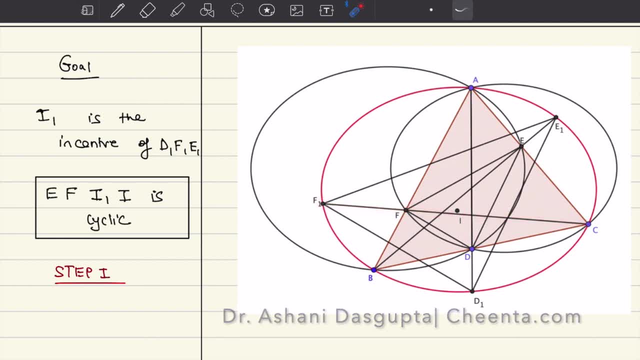 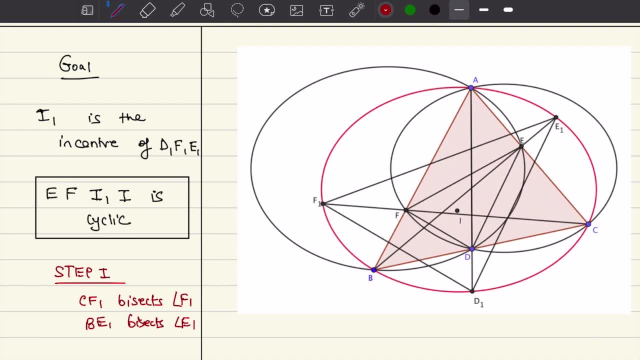 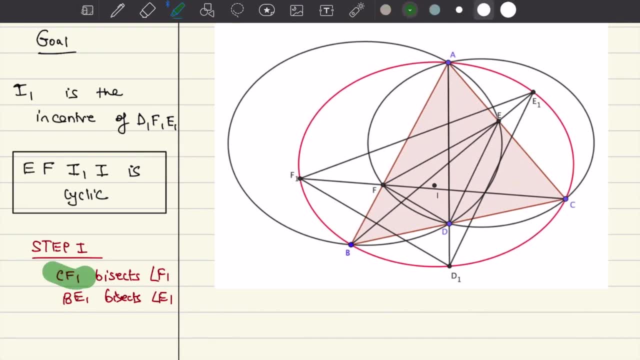 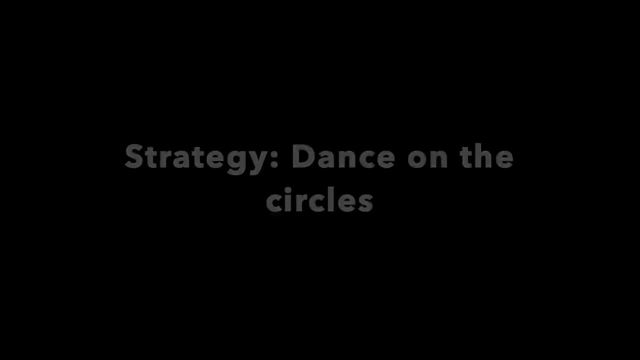 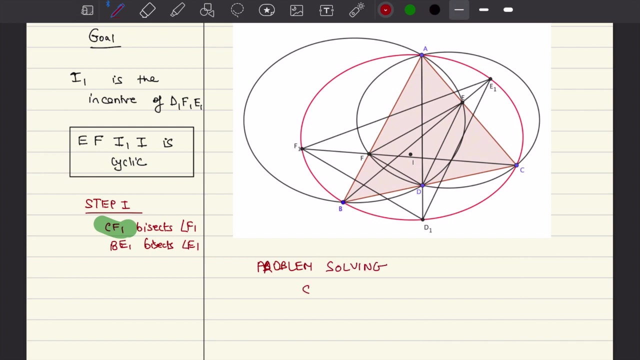 angle E1. now, why is that? well, I'll show you the first one and you can try the second one. so let's look at CF1. why CF1 would bisect angle F1? problem solving strategy. the strategy is this. I call it dance on the circles. 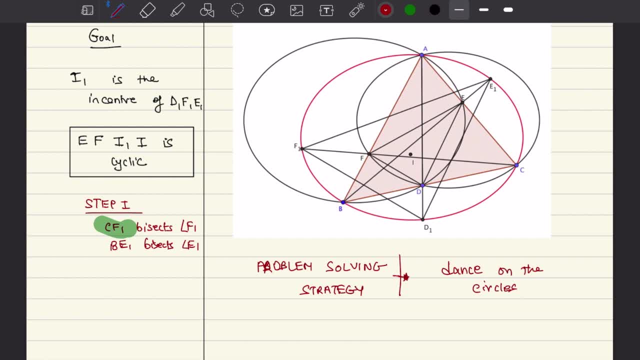 and believe me, that this particular strategy is actually useful for a multiple geometry problems, not just this one. so it's very important that you sort of learn this strategy. I call it dance on the circles. let me show you what it is all about. my goal is to show that CF1 bisects angle F1. to do that, I need to show that these two angles are. 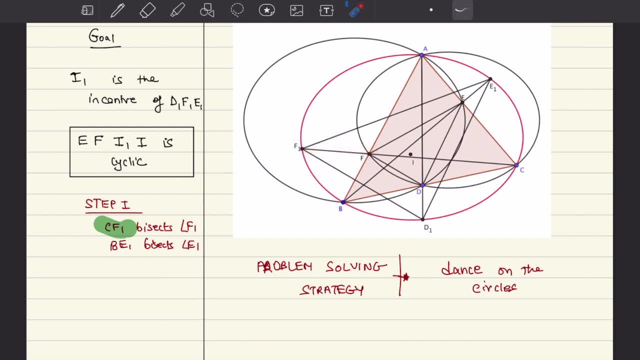 equal, of course, only then it will be an angle bisector. so what I'll do is I'll start with one of the angles- let's call it theta- and then I'll show you that the angle bisector is equal to the, and I will use properties of cyclic quadrilaterals to dance on these three circles. so one circle. 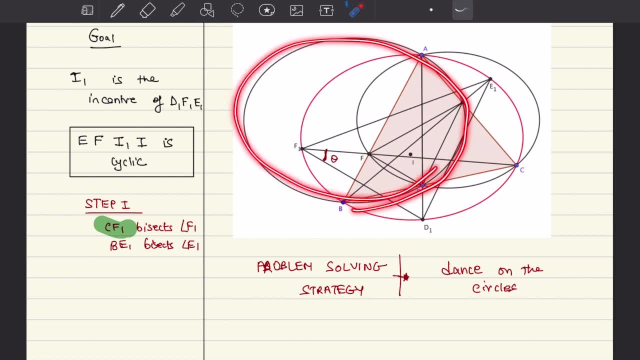 two circle and three circle. So let me show you how it is done. Let's first focus on this angle, theta. it is subtended by cd1 on the red circle. Now let's look at what other angle it is going to. so this is theta. cd1 subtends this angle on the red circle as well, so this is also theta. 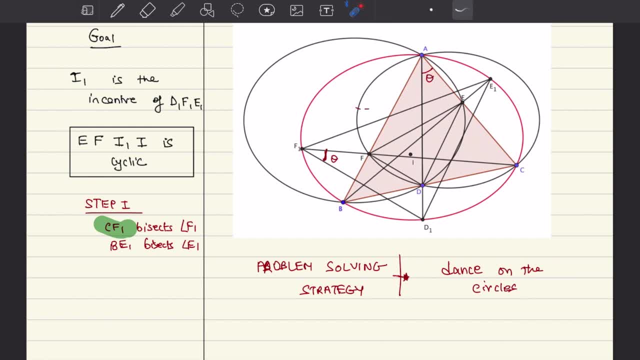 now, if you look carefully, this angle is also subtended by c ed arc on this black circle, right. So we now have. we have now switched to the black circle from the red circle, so this ed subtends theta. now let's see what else the ed subtends on this black circle. 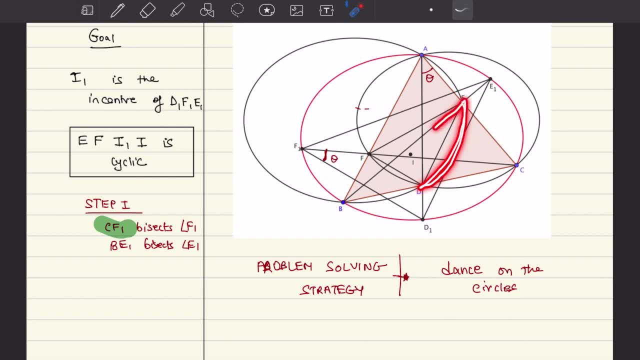 so ed also subtends this angle on the black circle. so this angle is oops, this angle is theta. now we dance back to the red circle. you see why i'm calling? i'm calling this the dance of the on the circles. so i dance back to the red circle, since this is theta, therefore, here this angle will also be theta. i have to join. 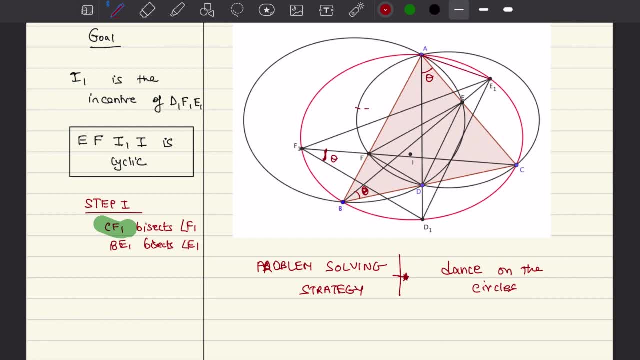 these two first, of course, so this is also angle theta. now one final time. i notice that this angle is theta and it is subtended by e1c, but e1c also subtends this angle at f1, so this is also theta and we are done. we are done showing that these two angles are equal. it's extremely important. 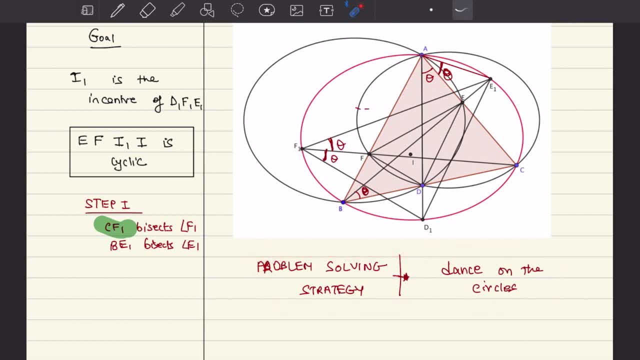 that you understand this strategy, this strategy of dancing on the circles, because it is useful in the knowledge of Samsung's PI75A. i've talked about that in previous lectures, but this is what you will learn this time. i'll us the data from this experiment: toardeflash, opening an. 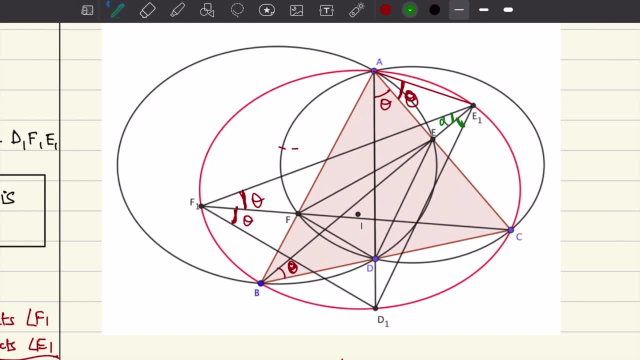 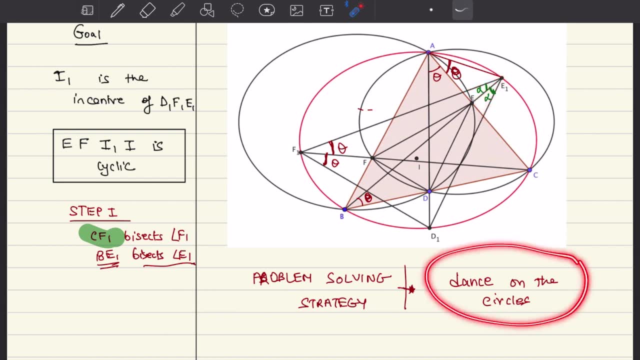 example, to compare it to the one i told you about wrong side axis and the answer here, and to lemon's~~~ may pi squared always comes cd for always single fla's. so it has to match the our mass over time, talvez, at least in our test. so this what we will learn in this day and today. 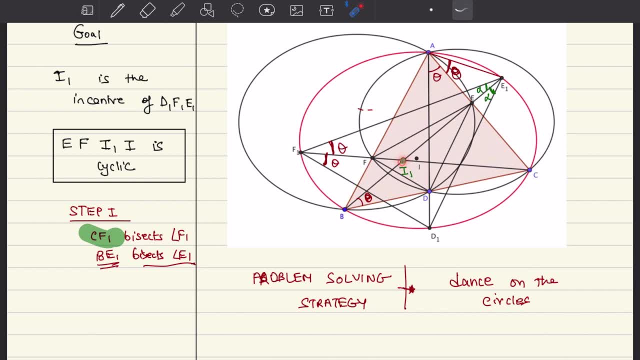 we will come to the answer for each of these problems. so if you are interested, please right click on the form and next slide. i will give you the example for the center of F1, E1, D1, because this is the angle bisector of F1 and this is the angle bisector of. 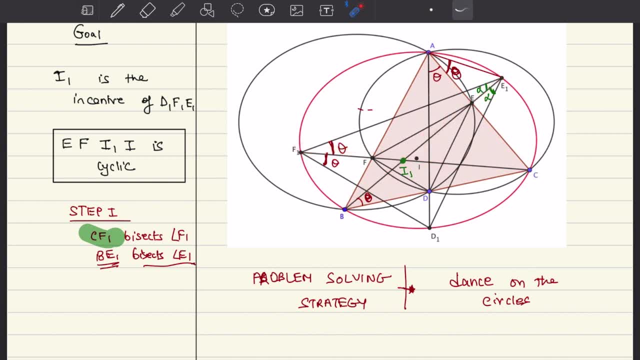 E1 and they are intersecting at the point I1.. Hence I1 must be the in center. Notice that if you do the dance on the circles, you will figure out that this angle is also alpha. In fact, exactly in the same way, if we join F1, this angle will also be alpha. 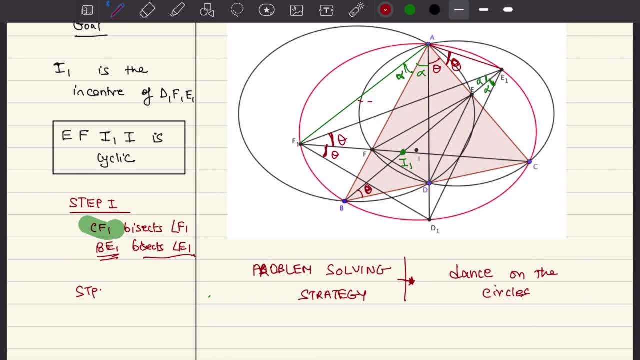 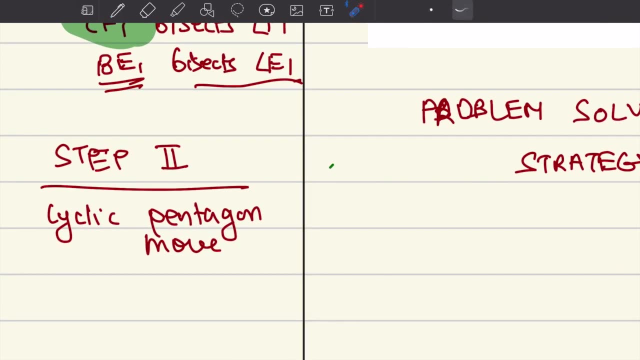 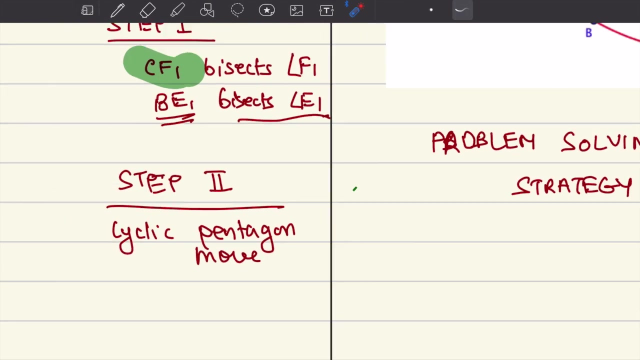 Now let's go to the step 2, and I call this step the cyclic pentagon move. Again, this is such a powerful tool, such a powerful configuration in geometry that you should definitely look out for it. So what is the cyclic pentagon move? 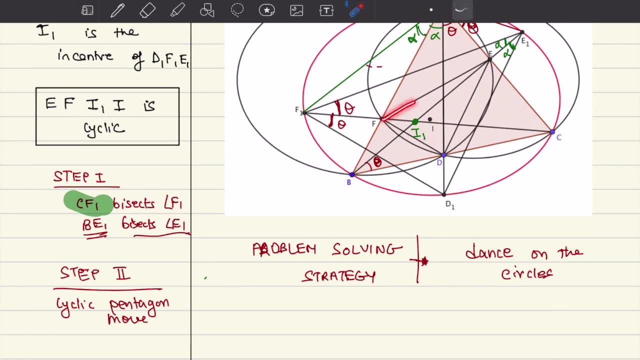 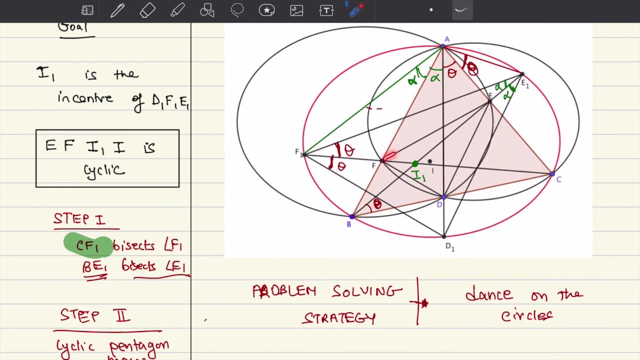 Well, suppose you want to prove that four points are cyclic. What you would do is you would take three of those four points and show that it is cyclic with some other point, Some other point- I don't know what point it is at the moment- but take three of those points. 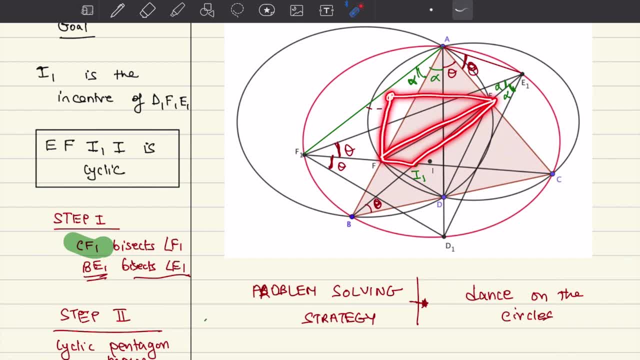 and show that it's cyclic with some other point, and then take other three of the points and show that it's cyclic with that previously held new point. So basically there are five points which are cyclic now and you get a cyclic pentagon. It's a very powerful strategy. 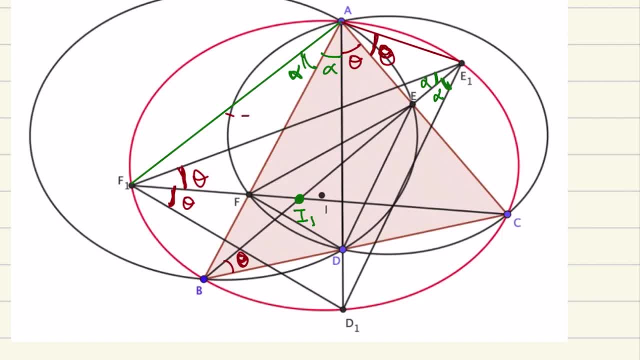 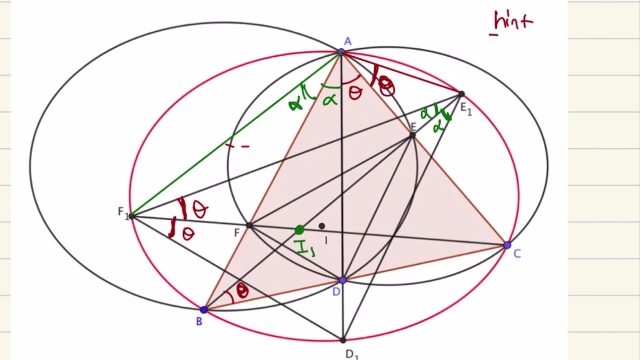 It is useful. It can be used in a variety of problems. So here I would say: the hint is this Hint and you can pause the video and try it on your own. Hint is: AFI1IE is a cyclic pentagon. Try to show that AFI1IE is cyclic pentagon. 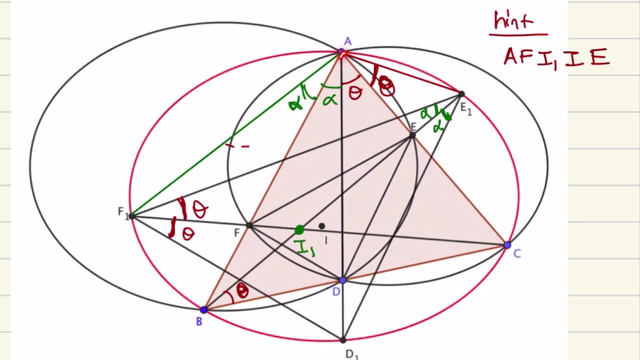 How do you do that? Well, first let's look at AFI1IE. This thing, Surely, since this is theta and this is alpha, this angle right here, in this particular triangle, is 180 minus theta, plus alpha In this triangle, if this is theta and this is alpha. 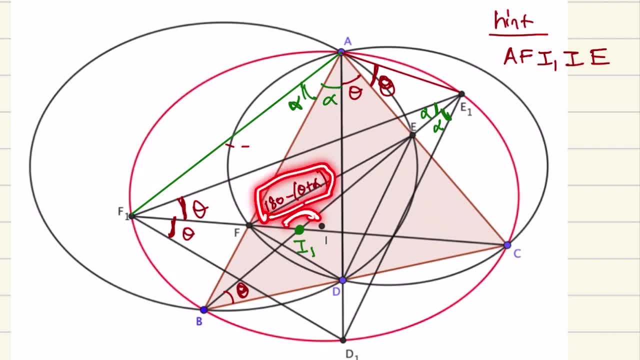 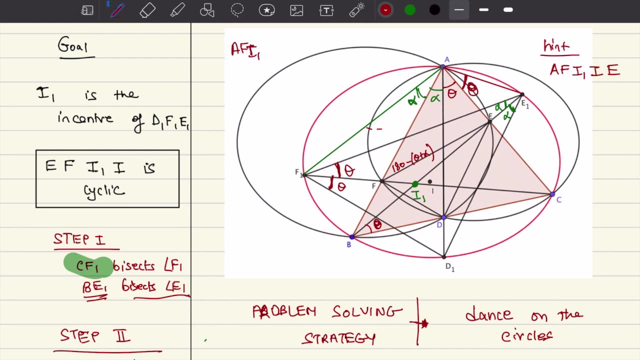 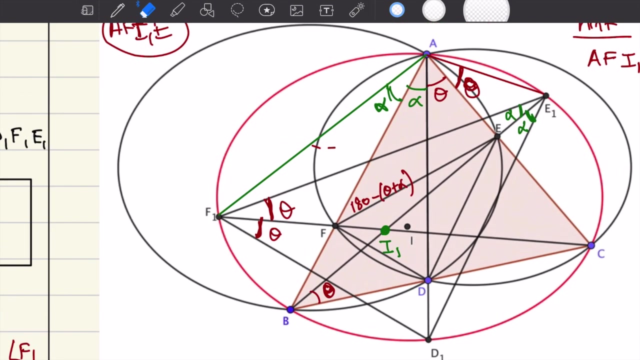 then this angle is 180 minus theta, plus alpha. So surely this is a cyclic quadrilateral. AFI1IE is cyclic. Okay, Now let's look at AFIE. Recall that I is the in-center of DFE. I is the in-center of DFE. 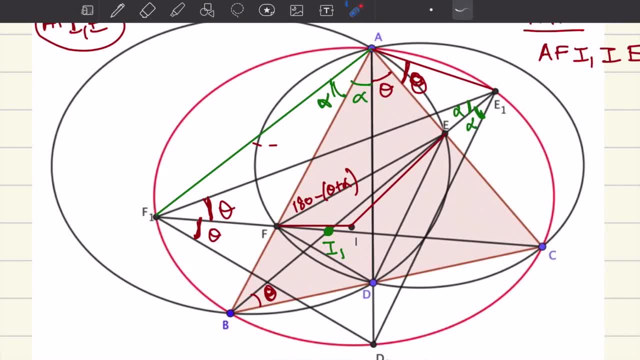 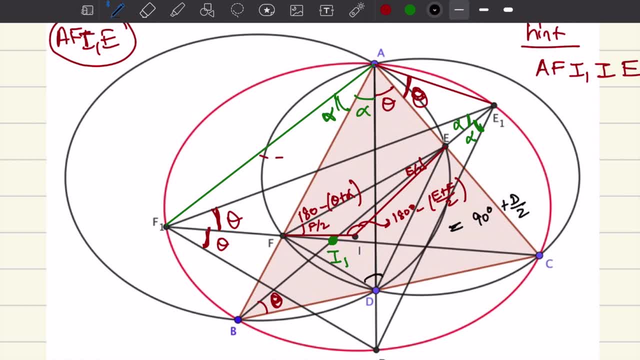 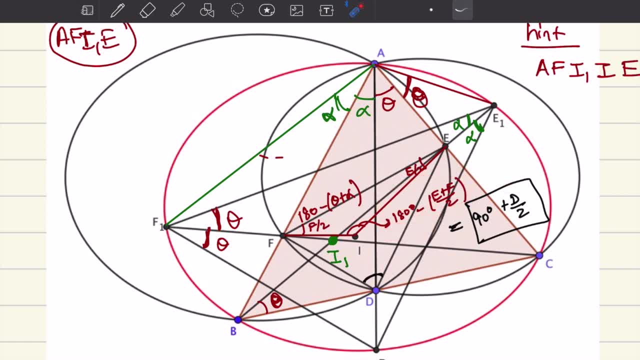 same as 90 degree plus d by 2.. Okay, we are almost done. Using the fact that this is a cyclic quadrilateral. a, f, d, e is a cyclic quadrilateral. we see that this angle right here is angle a, Because cyclic quadrilaterals have this property. this external angle is equal to the interior. 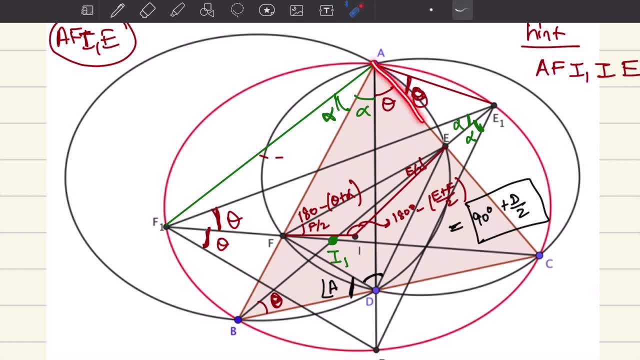 opposite angle. Similarly, since a, e, d, b is cyclic, therefore this angle right here is also angle a. Again, external angle is equal to the interior opposite angle. So clearly, angle d right here is 180 minus 2 a. So if you look at 90 plus d by 2, which was my value at angle i, this becomes: 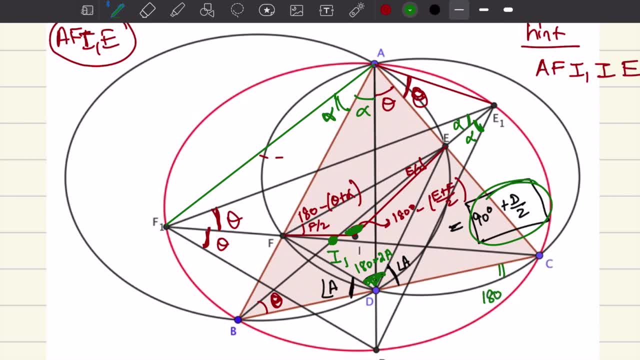 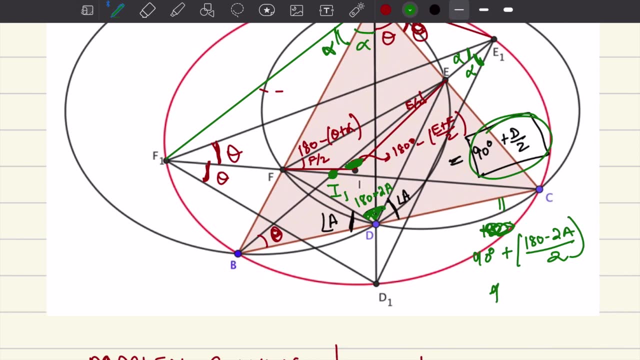 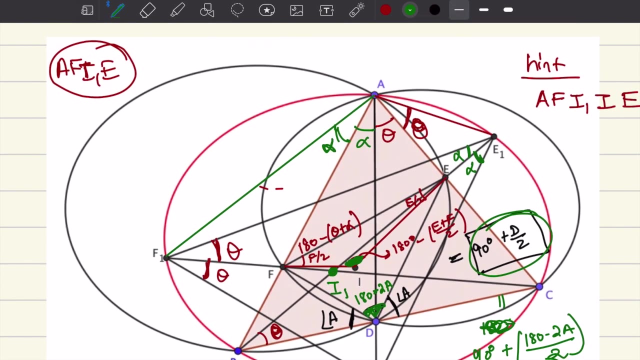 180 plus this becomes 90 plus 180 minus 2 a by 2. Which is simply 180 degree minus angle a. And that's exactly what we needed, because if this is 180 degree minus a, then this angle is 180 minus a and this angle is angle a, and together they 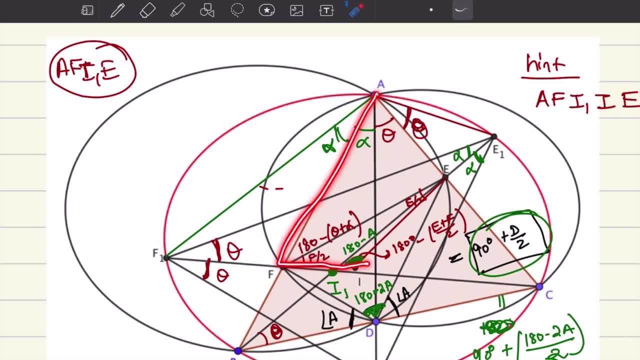 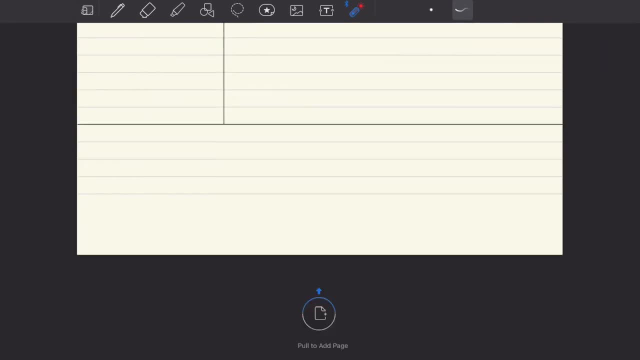 become 180 degree. So again we have a cyclic quadrilateral. So now then? now we have a cyclic quadrilateral That saying triangle for gradient mapping is 1 and left hand value coming from the vertical root of side oneöz and the right hand valuerites is 0, and this is a more simple